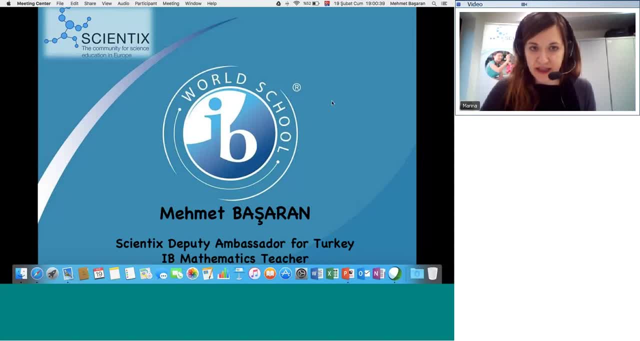 any difficulties attending the session. I would also like to remind you to please turn off your cameras and microphones during the talk and address your questions into the dedicated chat. So that's everything from my side. I will now give the floor to Mehmet. 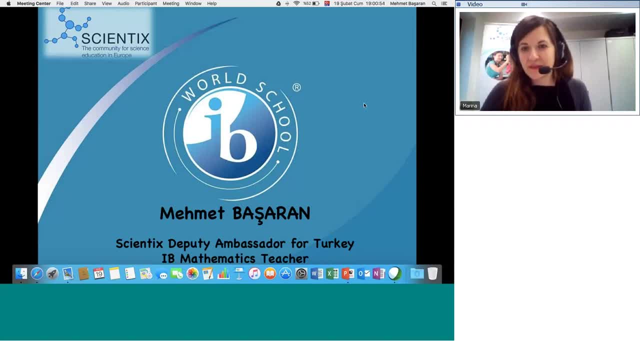 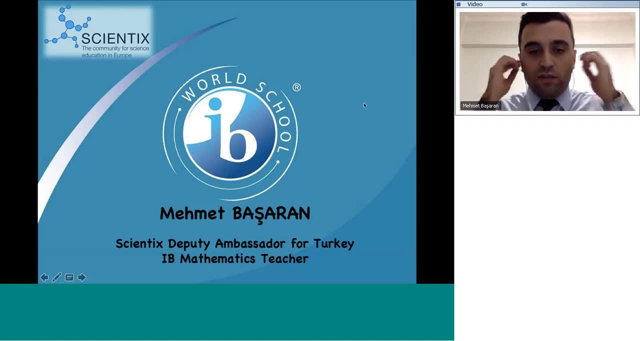 Thank you very much. Thank you, Marina. Hello everyone, I am Mehmet Başaran. Today we will be together and I will present you Scientix and STEM education and real world examples. How can we implement some mathematical topics in our mathematics lessons? And I will also give some details. 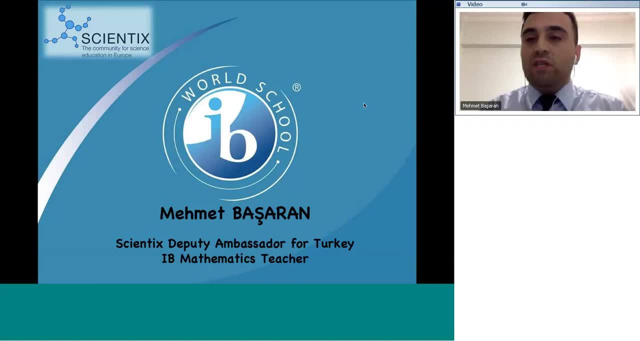 about IBDP program And you will learn about How we implement in IBDP program in our lessons. I will first start with the definition of mathematics, Then I will give some information about the daily life in mathematics Also, then I will give some information about IBDP. The last thing is, I will give some real world. 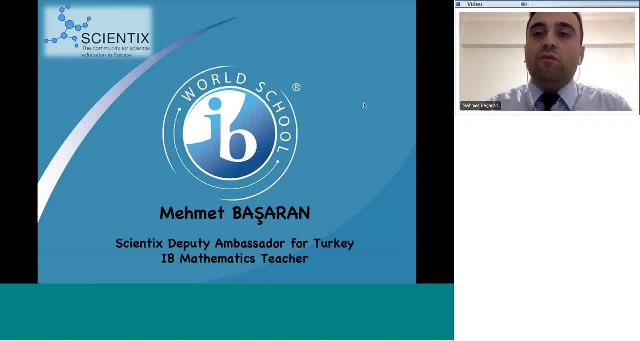 examples from lessons. Let's start with mathematics. What is the definition of mathematics? Mathematics is from Britannica. In Britannica concise encyclopedia is science of structure, order and relation that has evolved from counting, measuring and describing the shapes of objects. It deals with logical 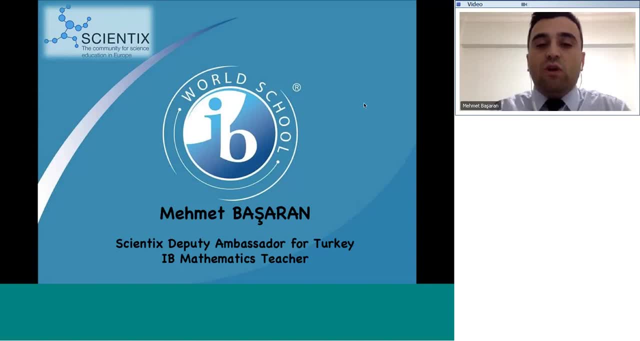 reasoning and qualitative calculations. As you probably see, here the mathematics is mainly about the logical reasoning and quantitative calculations And together with also literal meaning of mathematics is things which are not real. So we will talk about that in a little bit. Mathematics can be counted. Now you can think that counting has a vital role in our daily. 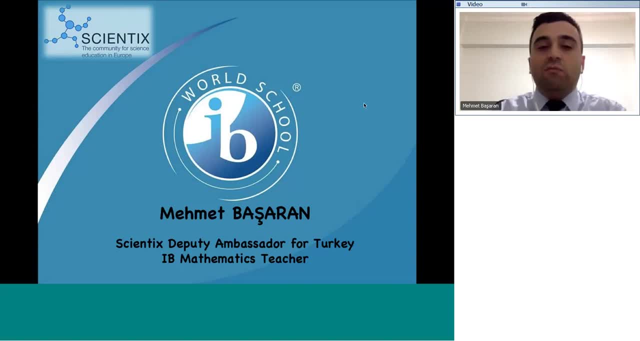 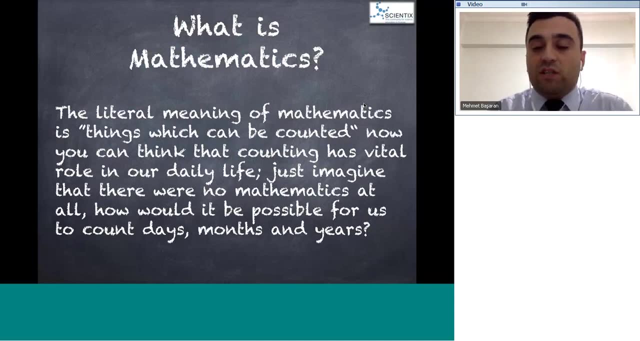 life. Just imagine that there were no mathematics at all. How would it be possible for us to count days, months and years? As you probably see here, maybe all of you know about what is mathematics. Let's start with how we use mathematics in daily life On a basic level. 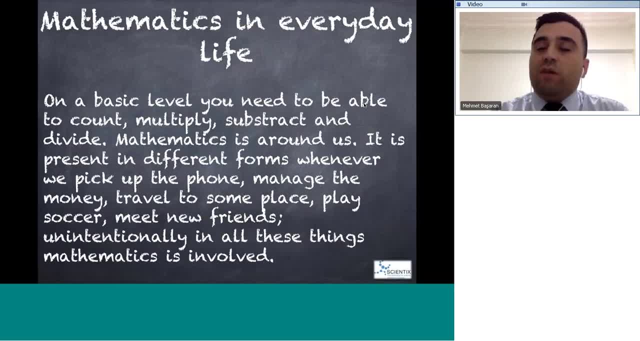 you need to be able to count, multiply, subtract or divide. Mathematics is around us. It is present in different forms whenever we pick the phone, manage the money, travel to some place, etc. meet new friends, unintentionally, In all these. 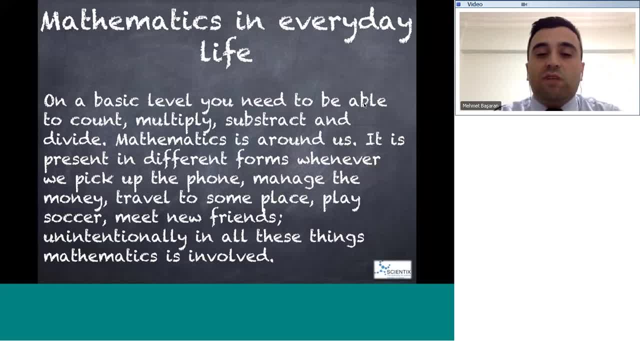 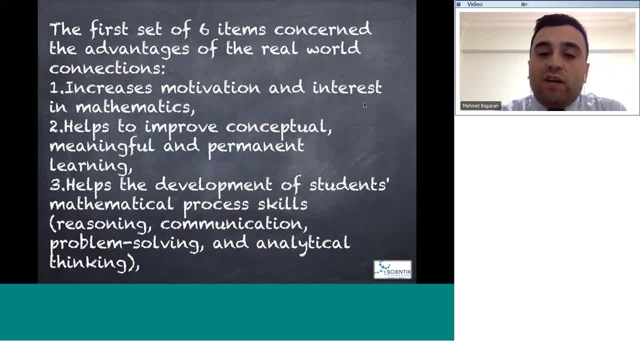 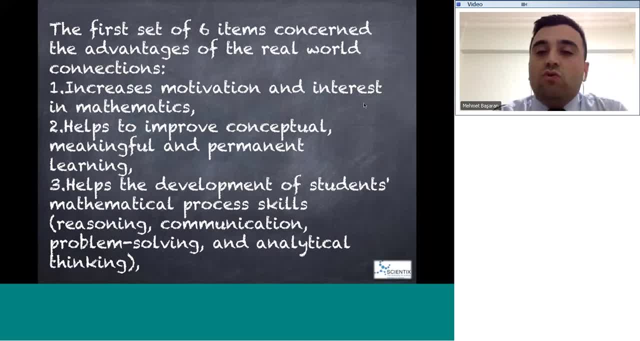 you do without real-world problems. The second thing is: real-world connections in mathematics helps students to improve conceptual, meaningful and permanent learning. In other words, students are more likely to learn from real-world problems than the. As you probably see here, the permanent learning is the most important part of all mathematics topics. 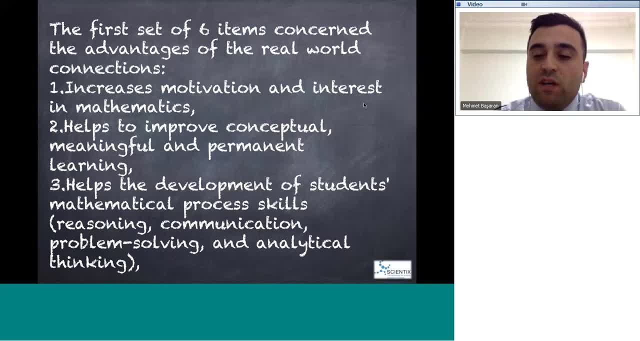 Probably all of the mathematics teachers deal with such problems And also making connections with real-life mathematics helps the development of students' mathematical progress skills, For example reasoning, communication, problem-solving and analytical thinking. Later we will see the IBDP program has parallel lines with real-world connections in mathematics lessons. 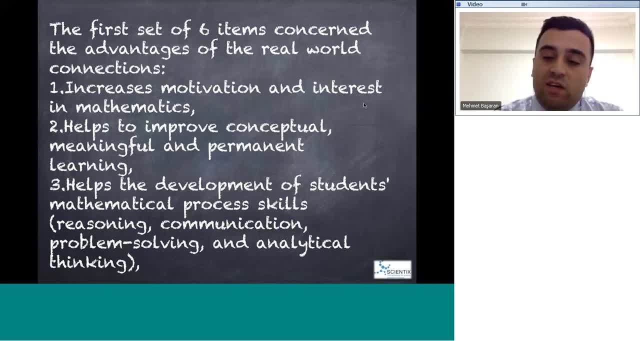 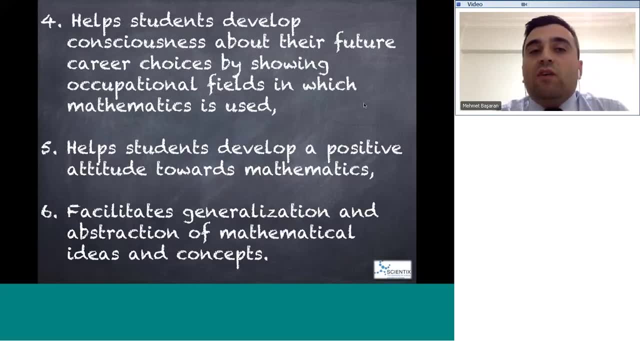 And if we continue with the advances of real-world connections. the fourth thing is help students develop consciousness about their future career choices by showing occupational fields in which mathematics is used. And the other thing is: real-world connections help students develop a positive attitude towards mathematics. 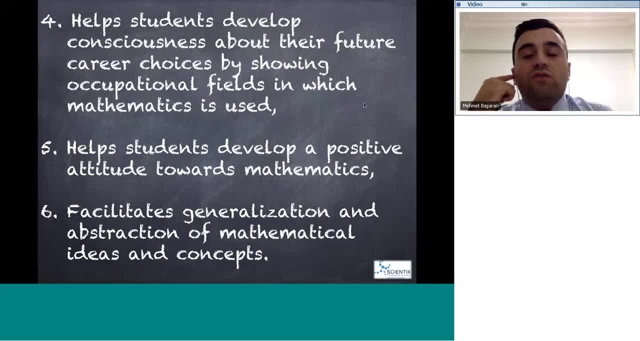 Probably, as you know, students have anxiety to learn mathematics Because if we don't have any connection between real-life and mathematics, how can they understand the mathematics? You know there are many research areas about it And I will also give some other important topics to connection with real-life and mathematics. 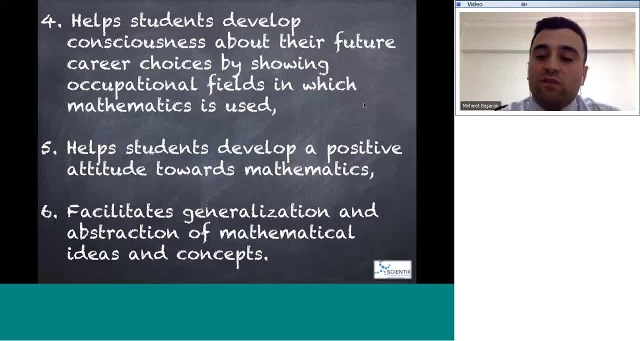 The third thing is: real-world connection facilitates generalization and abstraction of mathematical ideas and concepts. I give some important topics here because all these six things come from the research areas. You know there are many research about real-world connection and mathematics And you know I put together them here. 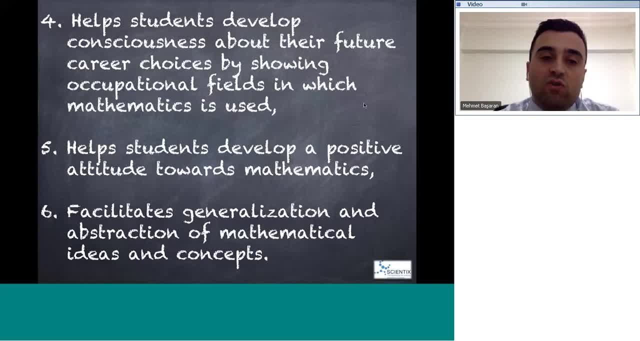 And I just wanted to give some information. Here are some important parts of them. But I really want to say here, if we just say the advances of mathematics and also I must say the disadvantages of what are, the disadvantages of the real-world connection and mathematics. 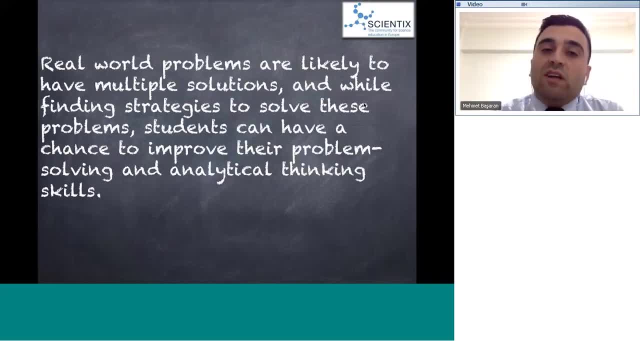 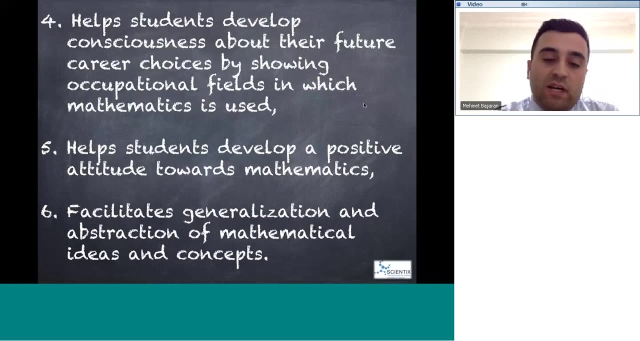 The first thing I would like to say: there is no significant disadvantage, But there are some disadvantages. For example, if given examples- given examples are complex to learn mathematics of problems can be difficult, You know, if we give difficult real-world examples. 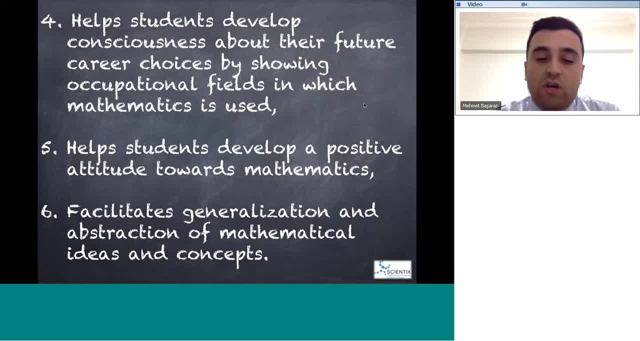 then the mathematics is become two times complex for students. Then also the other disadvantage is the heavy content of curriculum and lack of time may make it difficult to use connections. There are some disadvantages as you see here, And also you can guess them from your mathematics lessons. 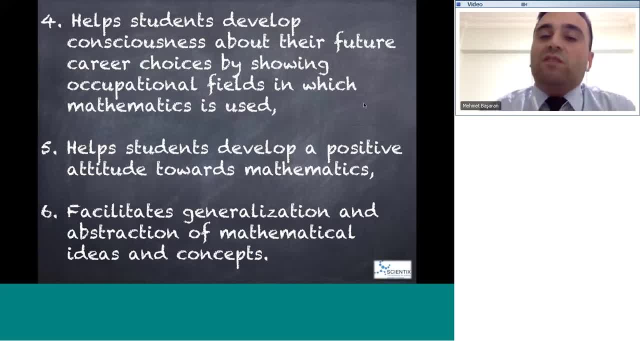 There are many disadvantages to use real-world connection and mathematics, But the research studies say that please use real-world connection and mathematics. I would like to continue with. real-world problems are likely to have multiple solutions And while finding strategies to solve these problems, 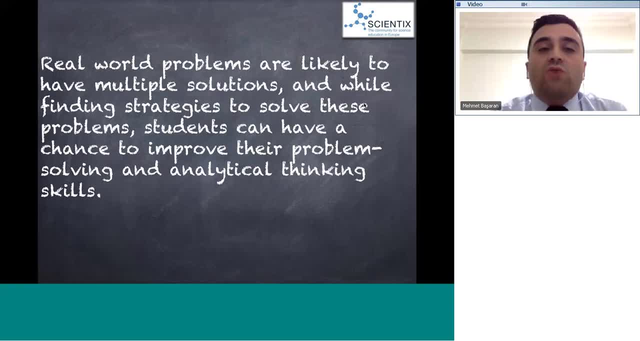 students can have chance to improve their problem solving and analytical thinking skills. As probably see here, if we connect the mathematics topics with real-world, then students will try to think analytically. Probably all of mathematics teachers want students to think analytically. 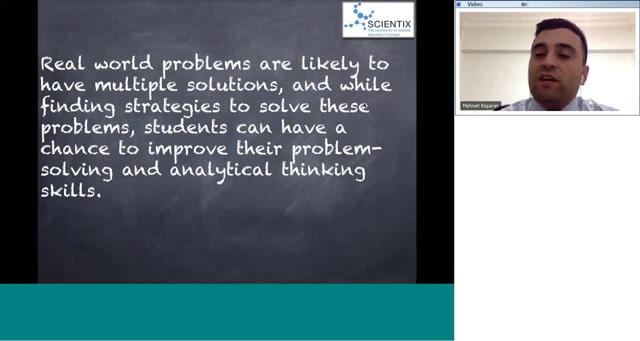 and have some skills, For example, critical, analytical and problem solver skills. That's why the reason: if we use some real-world connection in our lessons, then students will have chance to think analytically If we continue with the use of connections. 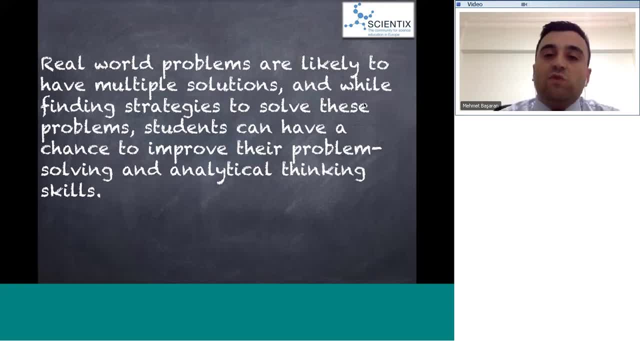 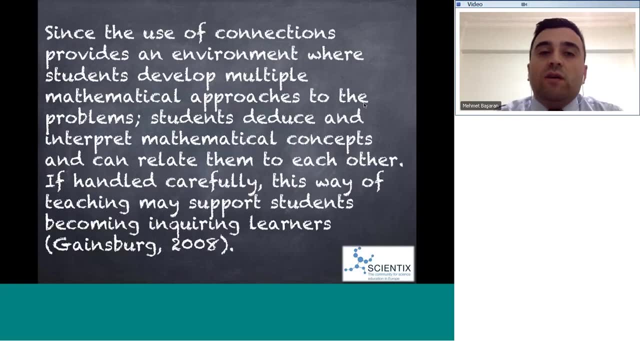 provides an environment where students develop multiple mathematical approach to their problems In this world. I would like to emphasize: if we use real-world connections, then we think about the differentiated learning. As you probably see, students have some different areas where they learn different types of problems. 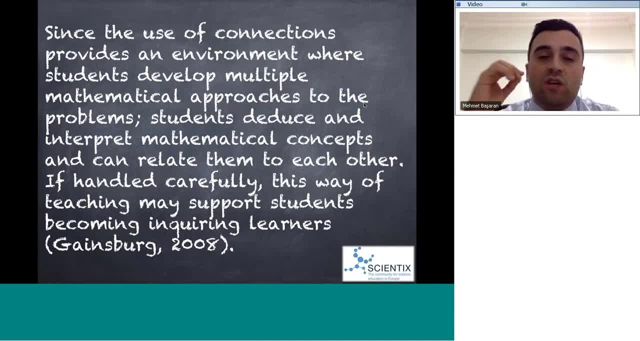 If we use real-world connections then we give them chance to solve the problems in a different way. That's why the reason the mathematics real-world connection gives us this chance and also students will have bigger chance to solve the problems in a different way. 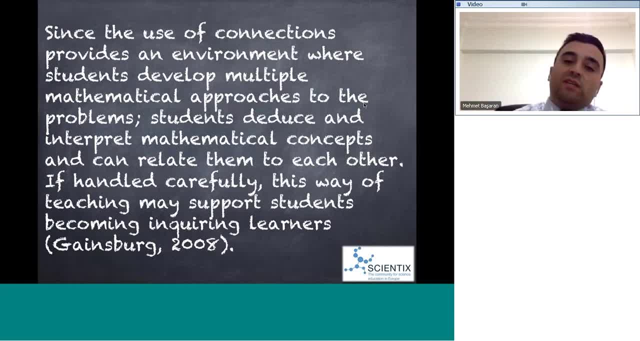 Let's continue. What is the IBDP program? Probably many of you heard about it, But here I will give some information about it I make PhD about in IBDP program and also I will give one example from the England Tenement School. 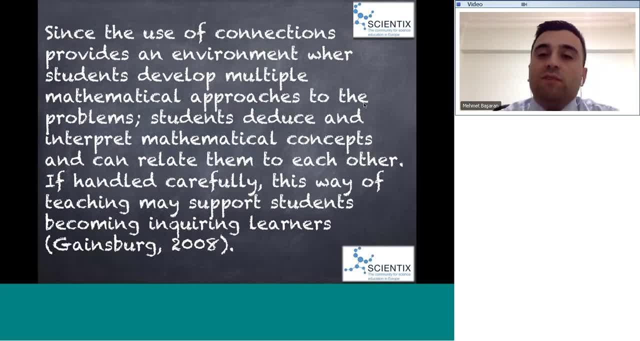 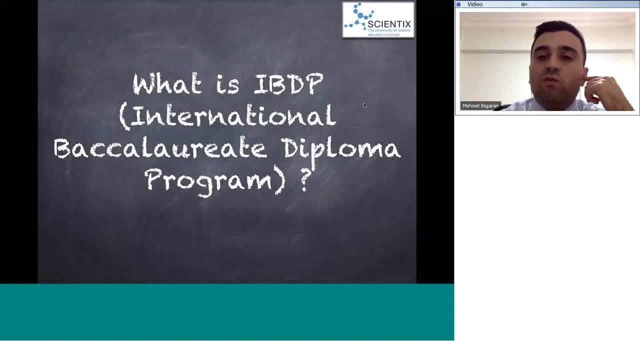 how we use mathematics connections in our mathematics lessons. First start with the IBDP. meaning IBDP has four programs. What are they? Primary years programs, middle years programs, diploma program and career related programs. Career related program is the newest one. 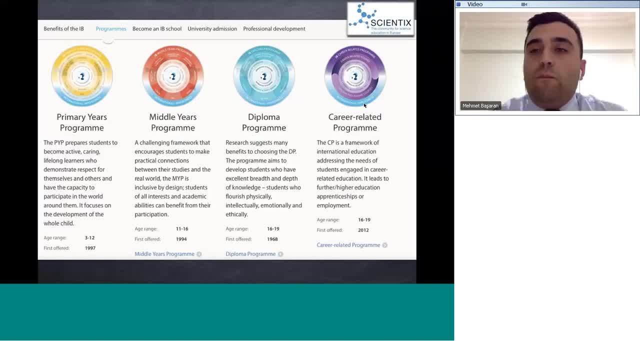 but I would like to hear mention about diploma program. Diploma program because gives students chance to go into university without an examination, because IBDP program has its own examination and students have more chance to study on IBDP program. Also, IB programs have more chance to students study other programs. 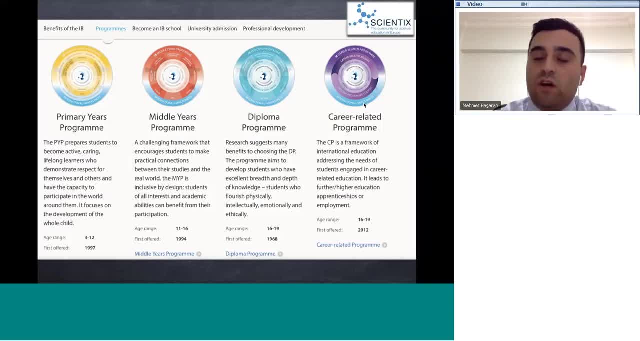 For example, IGCSE. IGCSE means International Graduate Certificate of Education or GCSE Graduate Certificate of Education. If students want to study on four of them, then students have more options in IBDP. My main interest in IBDP program. 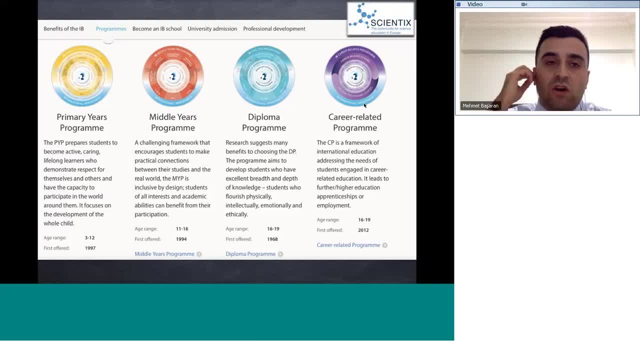 because I would like to study on diploma program to give chance to students to enter the university And continue. IBDP was established in 1968. The International Baccalaureate Diploma Program was the first program offered by IB And it is taught to students aged 16 to 19.. 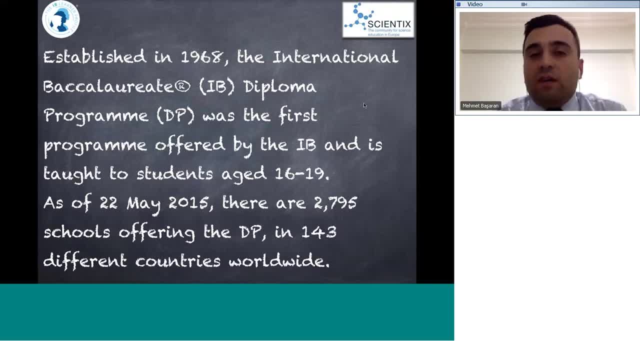 As of 20 May 2015,, there are 2,795 schools offering the DP in 143 different countries worldwide. As you probably see here, if you search on the internet, many prestigious universities accept IBDP program. Why I am mentioning here IBDP? 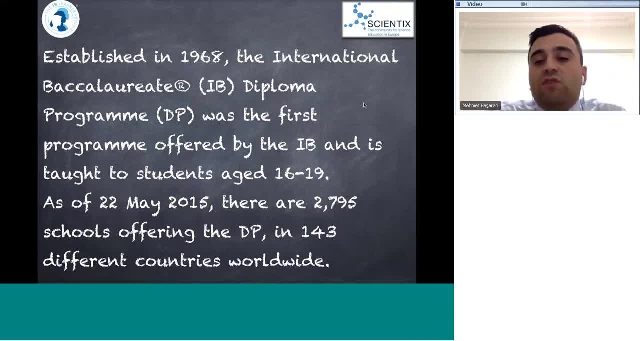 Because in IB classes we use real-world mathematics connections. IB calls these real-world mathematics connections is investigations in mathematics. You will see here the IB learner profile. IB learner profile is mainly about how we use the real-world connections Because IB wants students. 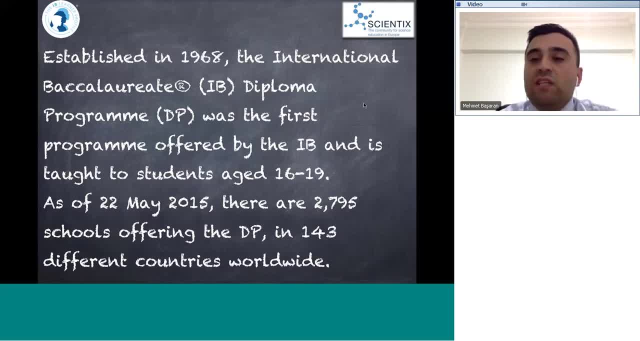 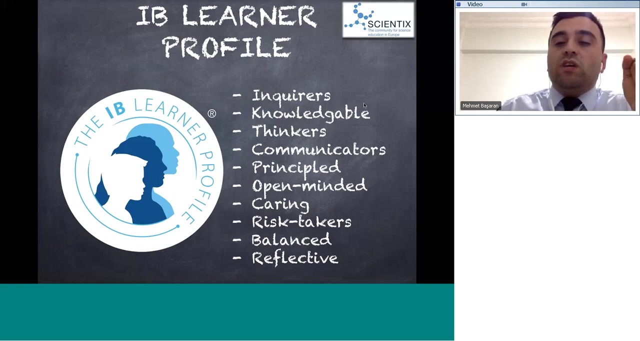 to be an inquirer, knowledgeable, thinker, communicator, principal, etc. You will see here, All these things is mainly about students must be on a holistic approach. As you probably know, the holistic approach it's mainly about the students must think. 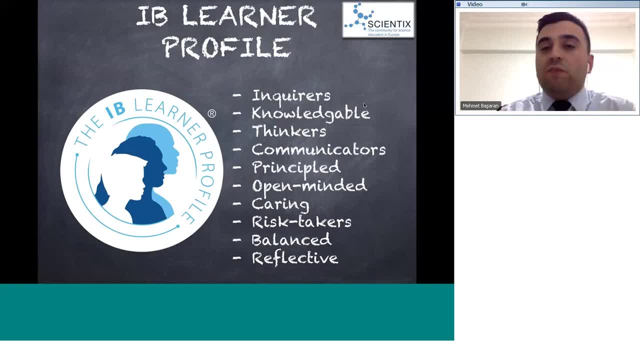 how can we connect the real-world and the topics from they learned from their theory of knowledge. And if you continue the assessment in IB, there are two types of assessments in IB. What are they? External and internal assessments- Two assessments: They are essays, structured problems. 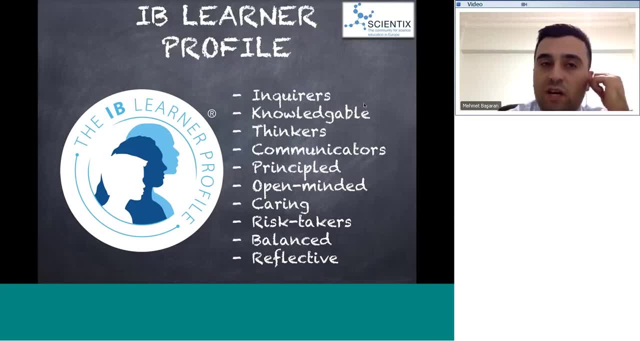 short response questions. data response questions. case study questions, Internal assessment, oral work, languages. investigations in mathematics. As you see here, students must study investigations in mathematics. They use real-world connections here. They also have more chance to use mathematics in investigations in mathematics. 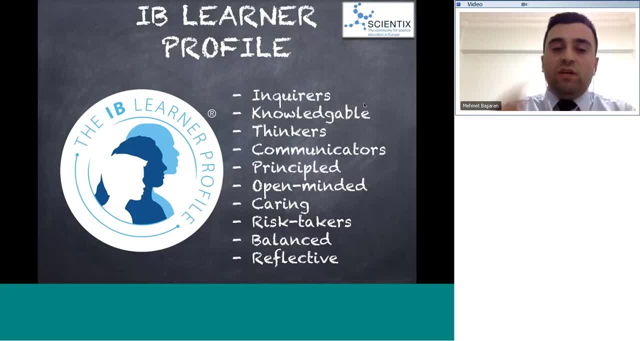 Also they must have artistic performance With the mathematics courses in IBDP. what are they? They are mathematical studies standard level, SL mathematical higher level and the further mathematics higher level. All these courses in IBDP mathematics courses. 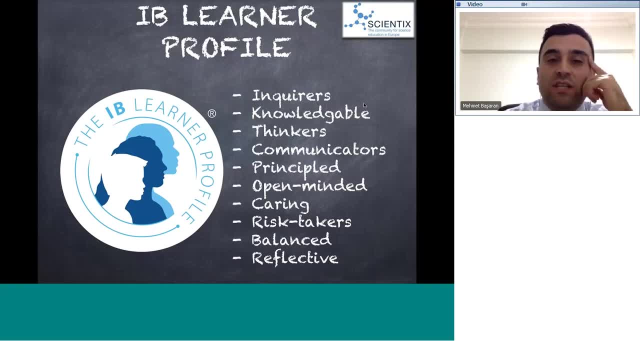 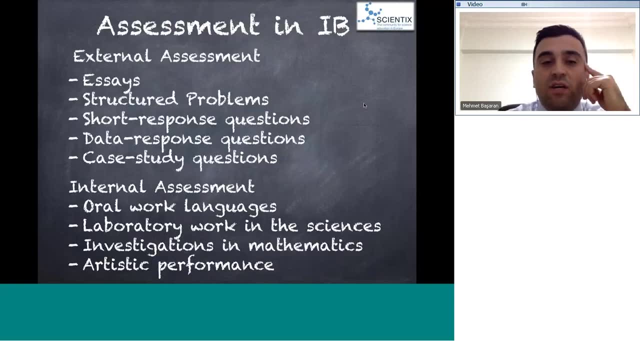 The aims of these courses are enable to students develop mathematical knowledge, concepts and principles, and also develop logical, critical and creative thinking and also employ and refine their powers of abstraction and generalization. As probably see here, students must think logically, critically and creatively because they have an exam. 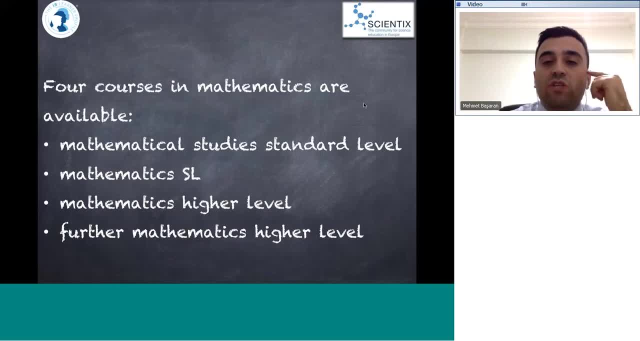 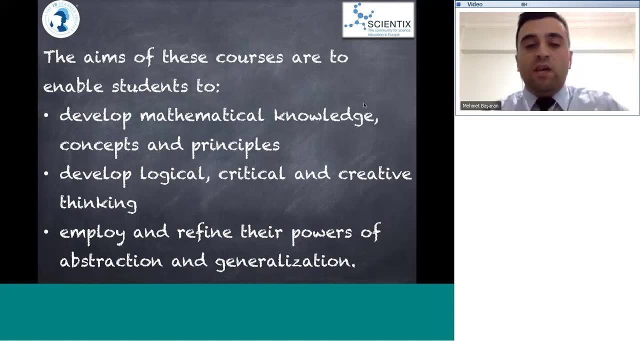 IBDP exam and also oral exam in their classes. That's why the reason students should know how they can connect the real world and mathematics. You know this is the big problem. Now I will give you some examples from the St Edmund's School. 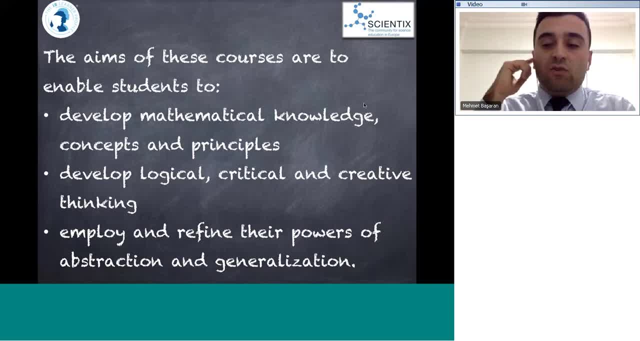 that I attend here as a student teacher. I will give one example how they implement their lessons: mathematics and real world connection. Here is the school. It's a very big area and very sophisticated. One of the lessons from this school- the mathematics lessons. 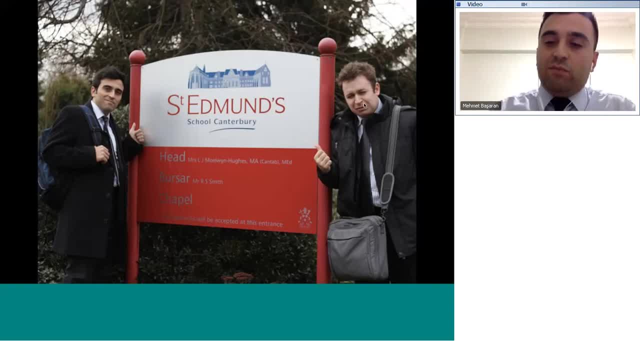 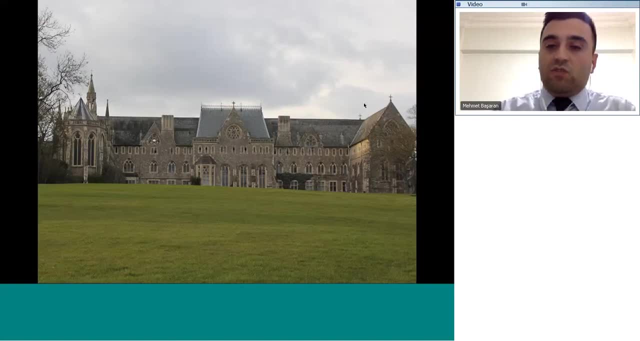 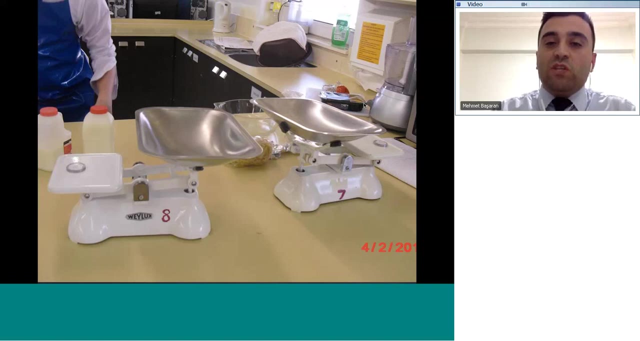 they use real world problems and also real world connections. First start with real world problem and the teacher gives them chance: Think about how can we solve these problems with using real world. For example, they should make a macaroni and they use kilograms. 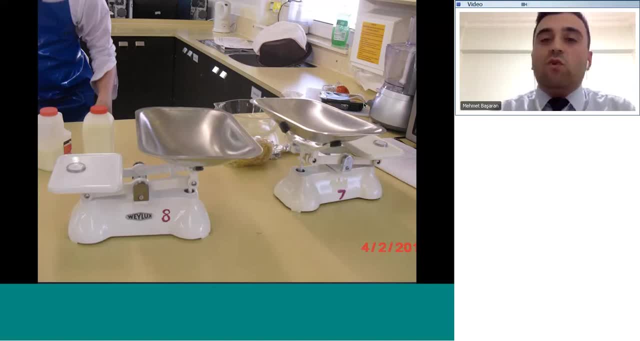 and other things and how they can put together them in one place and they must solve the problems in a suitable way. I will give you some examples here from the pictures. This is their lesson, mathematics, lesson that was interesting for me because in our country 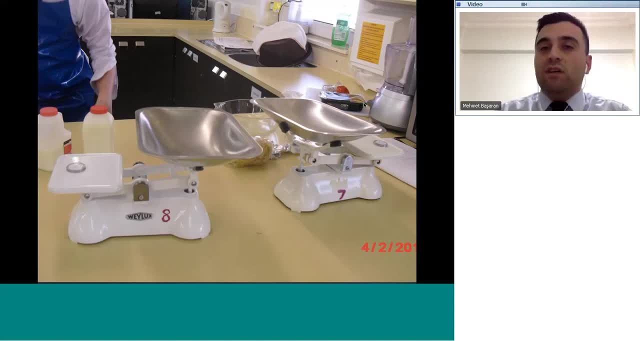 we don't use such areas to teach mathematics from the real life. They have more options here. This school was a private school. That's why the reason students had chance to cook the meals in a lab, as you see here, For example. this is the picture. 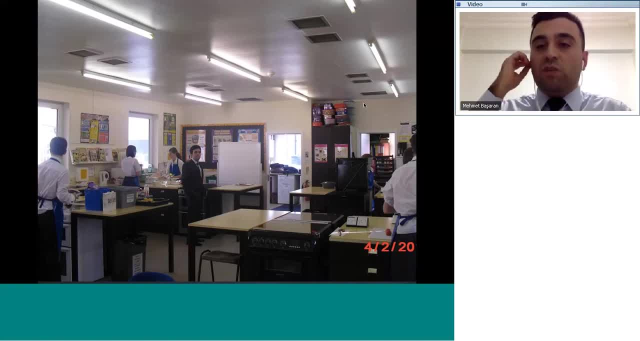 from their cooking. They first measure them and they must use the kilograms, and first then they must count, they must calculate. you know, probably you see here the real world connection and the mathematics At the end of the lesson they put on the board. 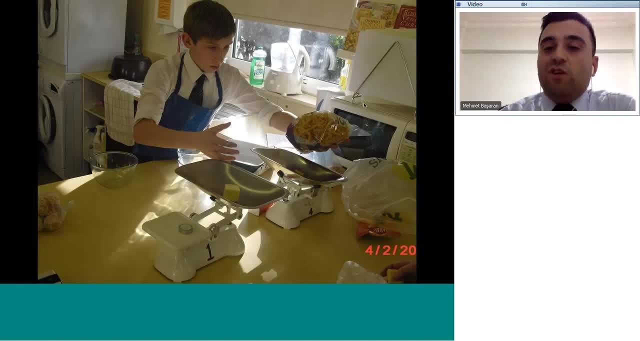 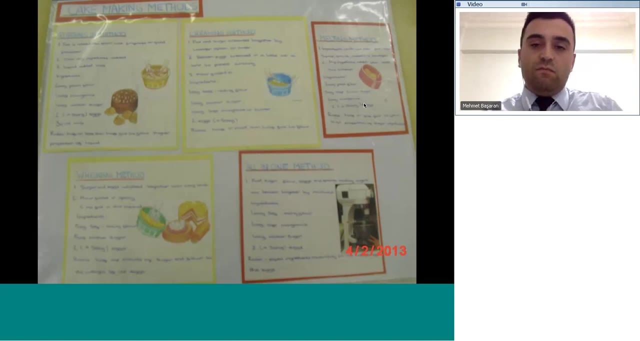 their writings and what they learned from this lesson. And here I want to give you one example from my IBDP class: how I use in my IB class mathematics. First I start with the real world mathematics. I ask my students: where do we use parabolas? 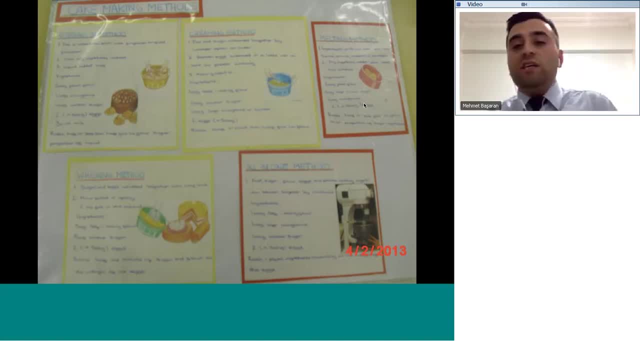 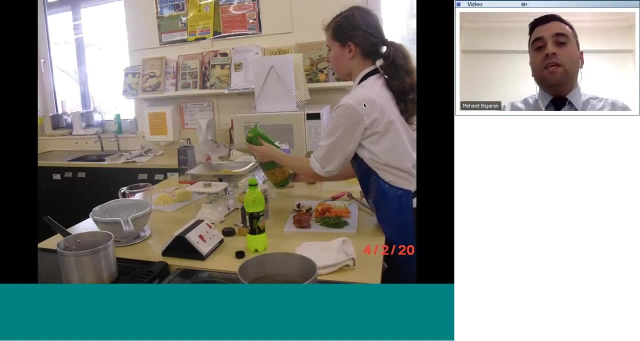 in real life. I come up with this question and I wait the students to think about it: where can we use the parabolas After discussion, 5 or 50 minutes? I give some real world examples from parabolas, For example. 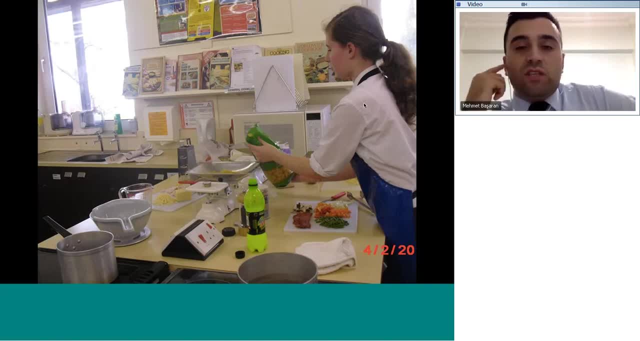 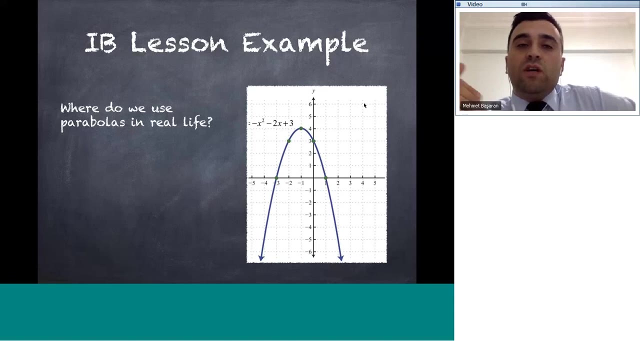 we use parabolas in McDonald's, For example, in the nature. probably they saw these things, but they had never thought this is a parabola. or how can we write the equation of this parabola? I come up with these such things to think them. 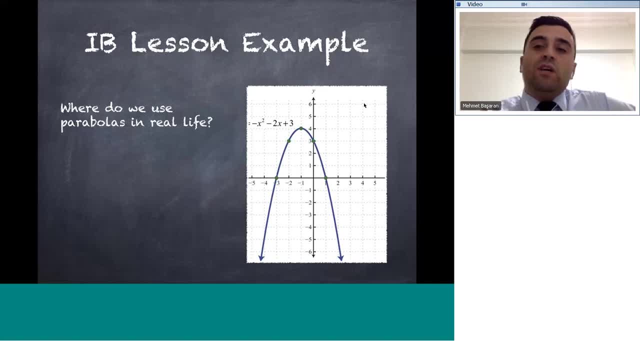 critically and analytically. And also I give some real world examples because giving more examples I visualize them, the abstract thinking and go beyond it. you know probably you have deal with to write the equations of a parabola because it's too difficult for students. 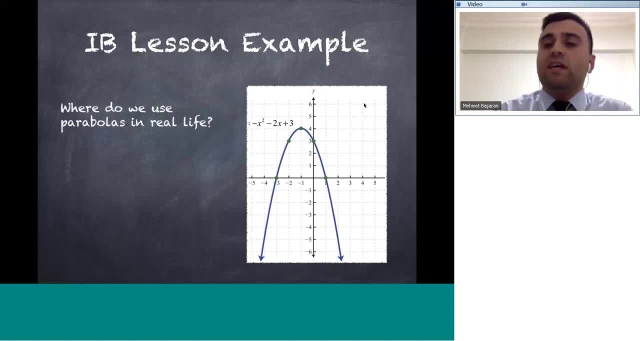 thinking first abstractly. If we give chance them first real world examples, then they will think: yes, we use the parabolas in real life and how can we write these equations? And then I give more examples. I every time try to prepare. 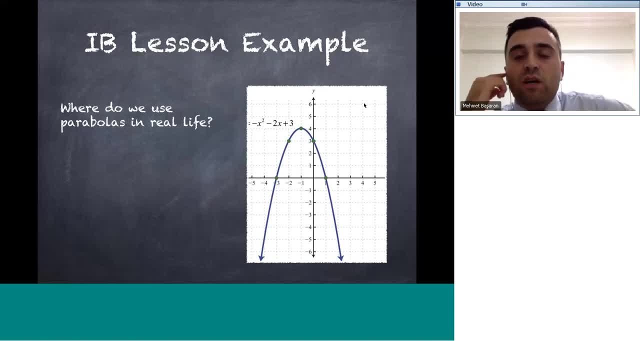 before my lessons. I know this takes time, but actually I must do this because I want to teach my lessons in investigations in mathematics. So I also give real bridges and they use the parabolas and the equations, For example here and here: 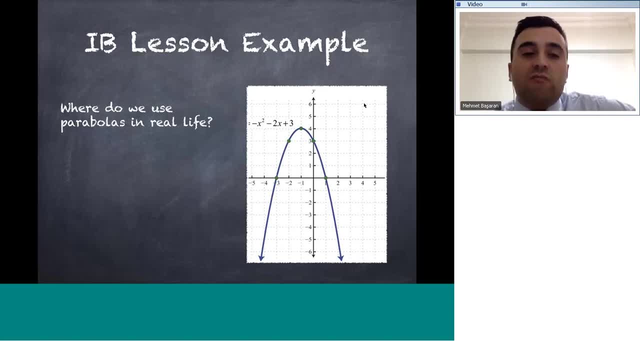 Giving more examples, you know, After giving these examples, and I ask my students: how can we write these equations? Yeah, you saw these problems and you see these real world examples and how can we use to write the equation of this parabola? 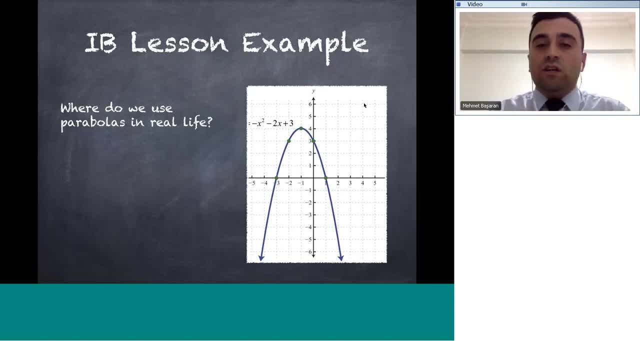 Students in IBD. they have more chance to write it because they have many options, For example, TI calculator. TI calculator gives students more chance to write an equation, what they have. For example, they can write an equation of the parabola. 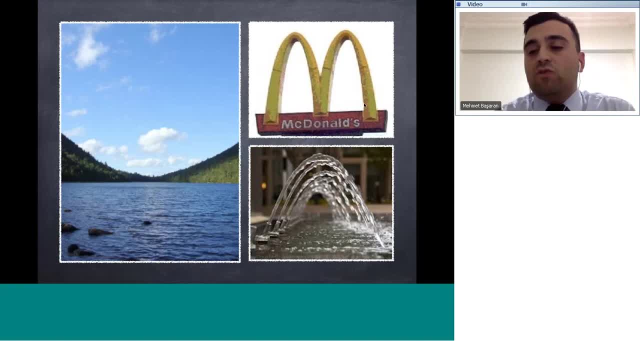 or other things. They know how to write in an equation in this TI calculator Also, they can also use the GeoGebra program. Many times I use GeoGebra program because it gives me more chance to make real world connection and to write the equations. 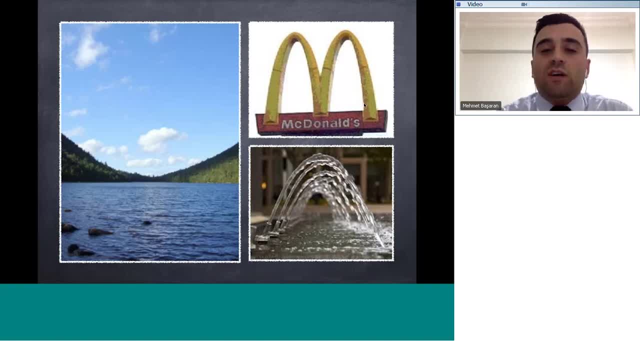 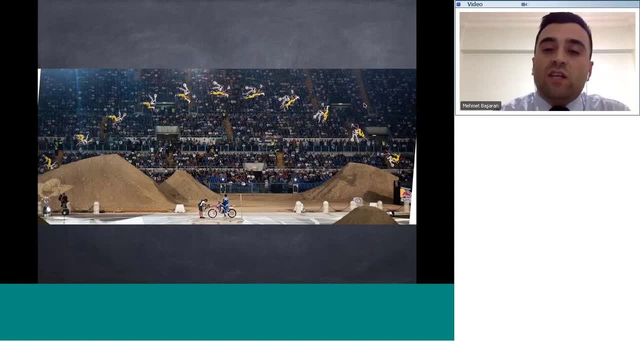 in a different way Because in GeoGebra program there are sliders. that gives me chance to move the equations left, right or upward. That's why the reason sometimes I use GeoGebra program. Students also know how to use the GeoGebra program. 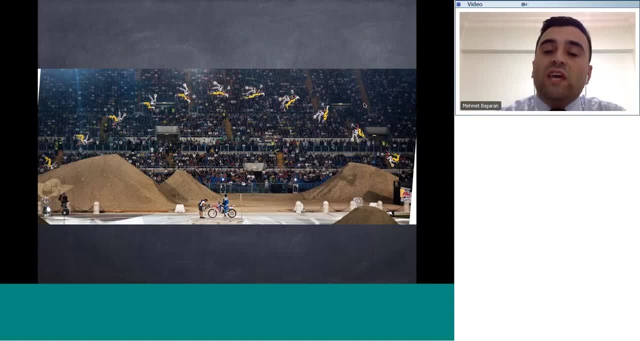 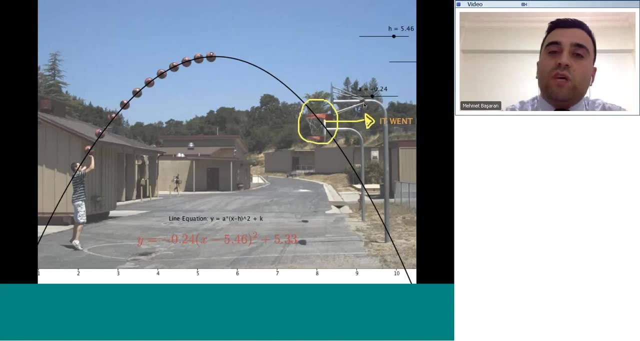 too. You know GeoGebra program is a little bit different from other programs. You know GeoGebra program is a little bit different from other programs. So you know giving some examples in our mathematics lesson students will come up. 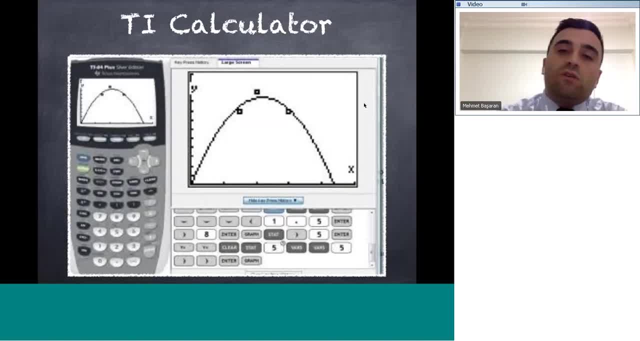 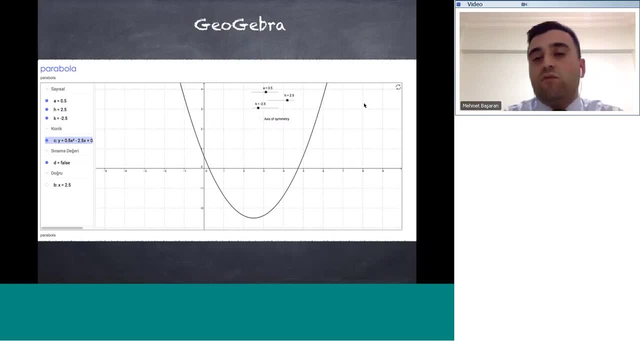 with you. Then how can we use the limits, or differentiation or integral? How can we use in real world and how can we write the equations and such things with using the technology? That's why the reason in our IB classes we sometimes use 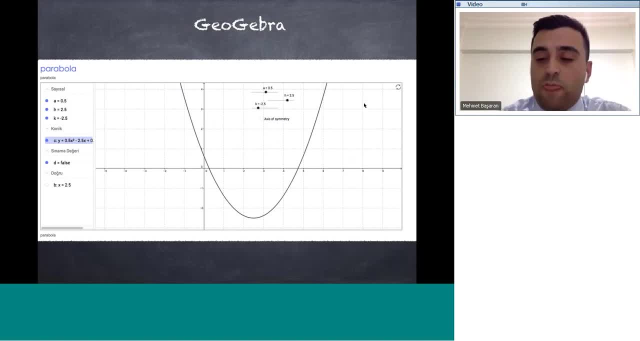 such things, but sometimes we don't know how to use such things. So in our MAB classes we don't use such things because, you know, our students must study for their university exam, They must solve many different questions. They must use 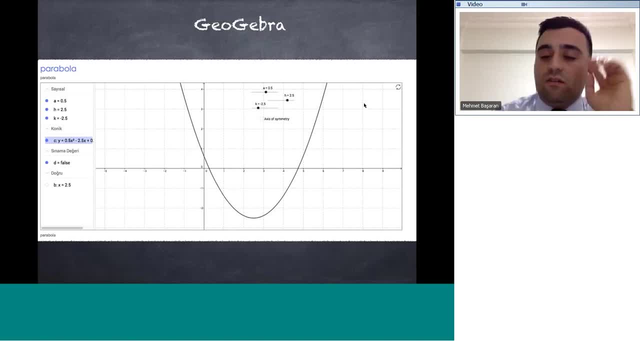 different solving styles In our in my country using mathematics is a really big problem because they must solve many, many different problems in one minute for just one mathematics question. But in IB classes I have more chance in our in our country. 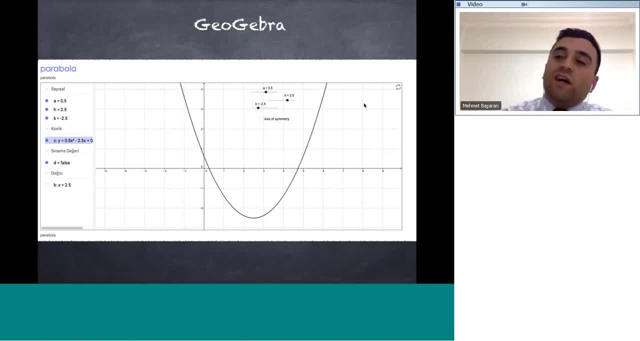 this is the new thing you know using mathematics and real world connection. Probably you use your real world connection in your lessons, but in my country this is so difficult. But actually I had a chance in Belgium, England. 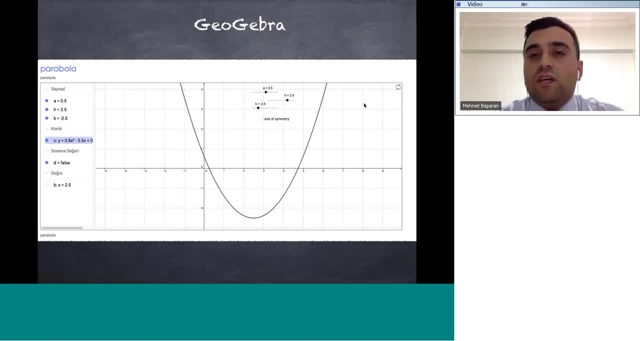 and France and such countries use real world problems and mathematics because they really want to think the students critically, analytically. you know, these are the 21st century skills If the students want to move higher and if we want students to go beyond. 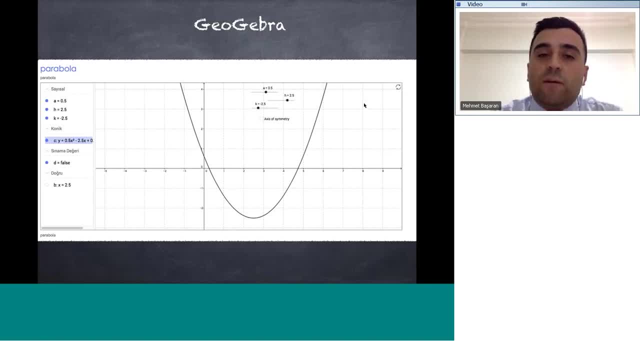 we must use in our mathematics lessons such mathematical topics. Finding some mathematical topics from the real life is rather difficult, but I should advise you: please try to find different mathematics topics for your teaching lessons. This is my presentation. If you like to ask some questions. 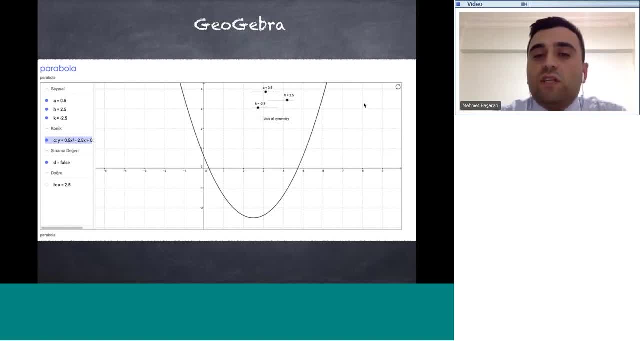 please ask me. Thank you everyone, Hello, Hello Hi. Thank you, Mehmet, for this presentation. We do have some time for questions. I don't know. if anyone wants to share something in the chat, Feel free to share. 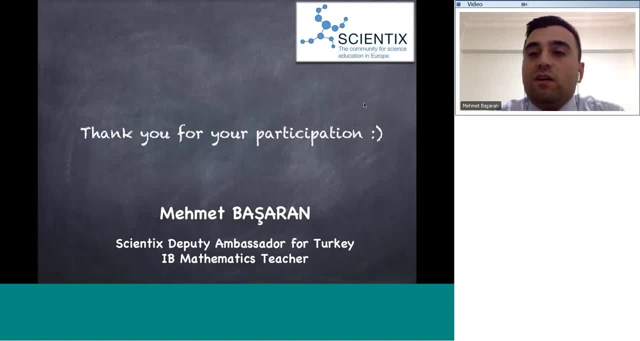 it now, But I can't see anything in the chat. Would you like to expand on any of the topics that you have mentioned, maybe? Okay, I can if I have a chance. I would like to give some websites about real world. 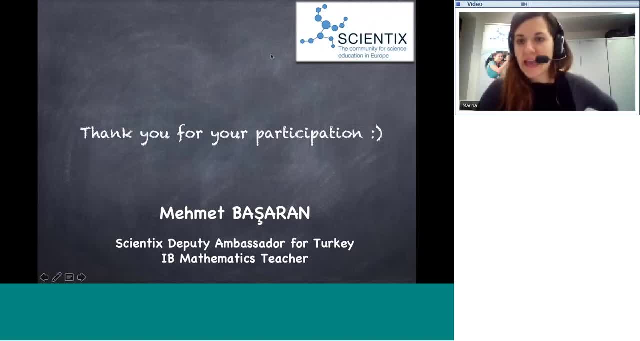 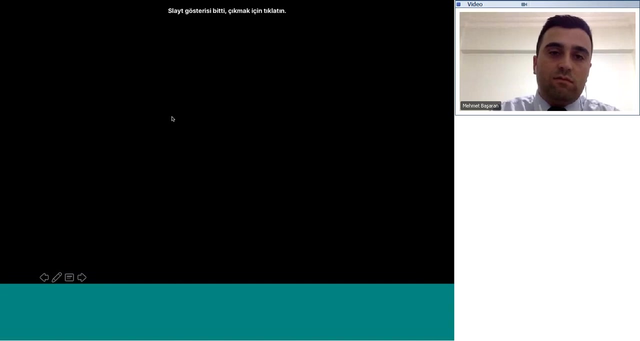 connections to find the teachers I would like to give them. Yeah, Here are some useful websites for using Pumas: practical use of math and science. Here you can use different kinds of mathematical topics and real world connections. You can click one. 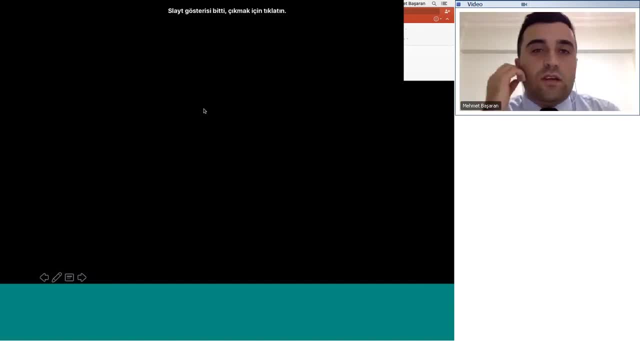 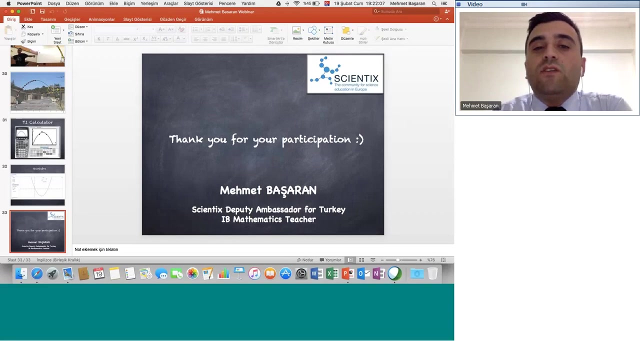 of them and you can find the real world connection. For example, how big is the Earth? I use some in my lessons And other things. the math in real life you can use in your lessons here. You know this is a great. 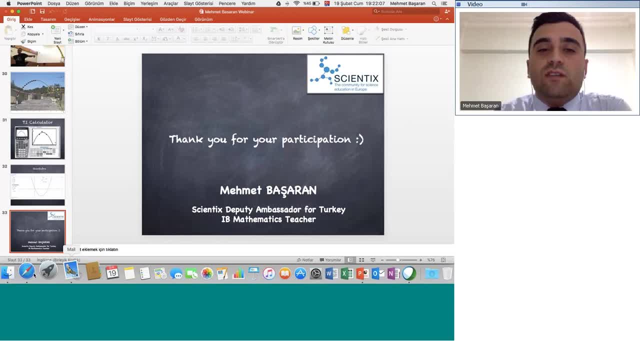 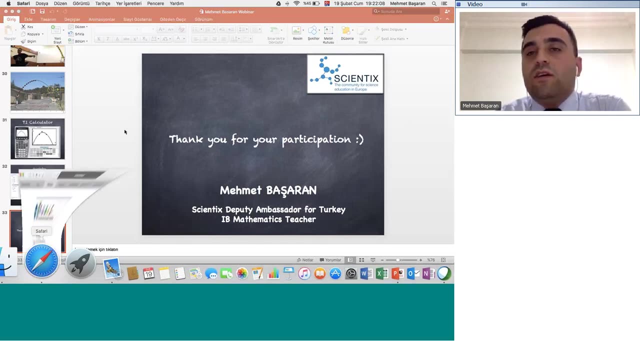 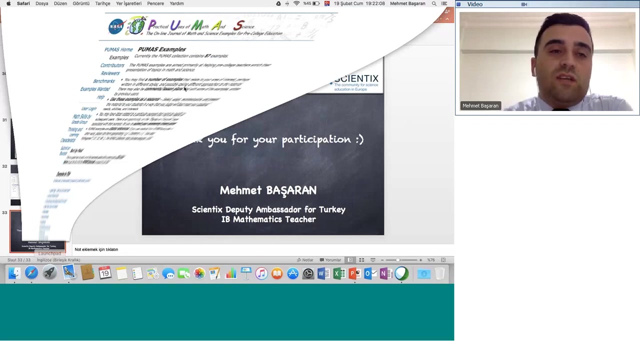 example of mathematical websites using real world examples And other things. math motivation I also use here and also you can use some math videos here. Mehmet, sorry for interrupting, but we're seeing the video very slow, so when you're. 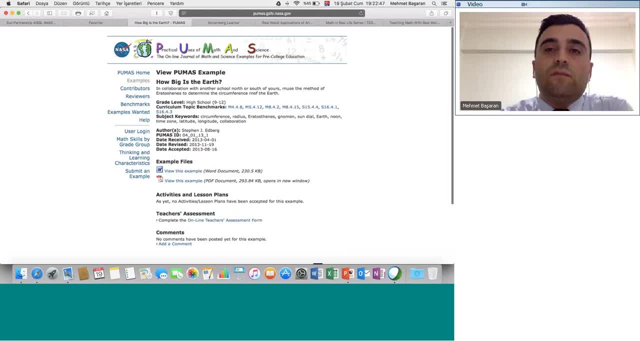 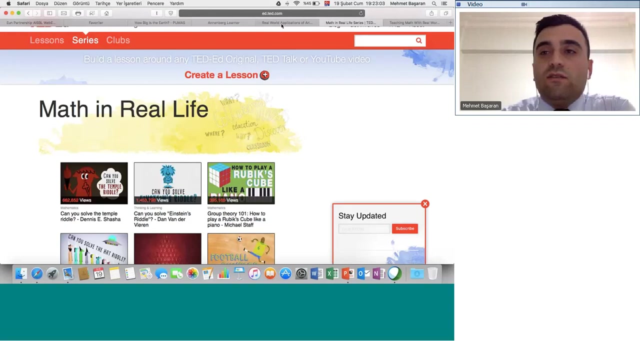 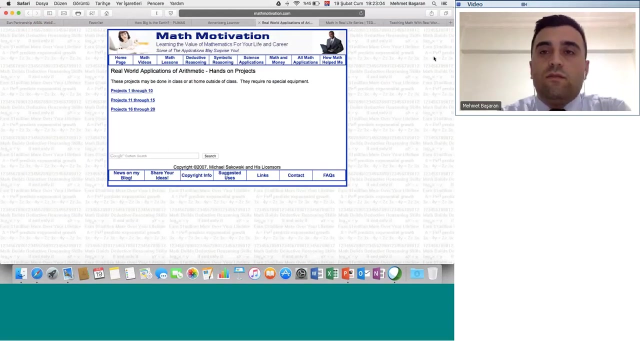 talking, we still don't see the pages. Okay, I am waiting. Yeah, thanks, Do you hear? now We can see it now. Okay, Here another good example of website using mathematics in real life. you can use these mathematical. 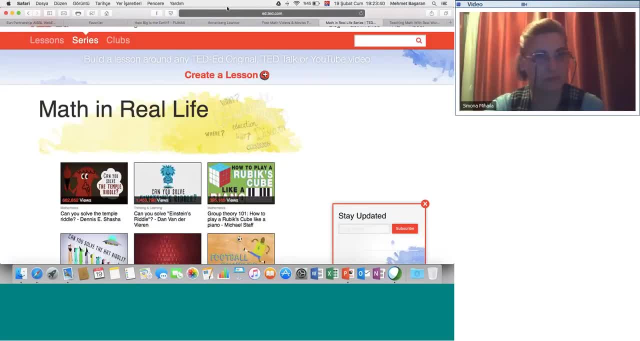 topics here. You can choose one of them and you can arrange. also, But mostly, I use the Pumas and some examples math lessons to motivate the students, to hook them before the lessons starting your lesson. Also, you can give some teaching. 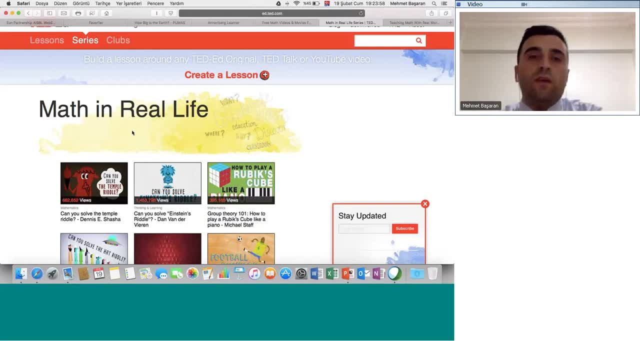 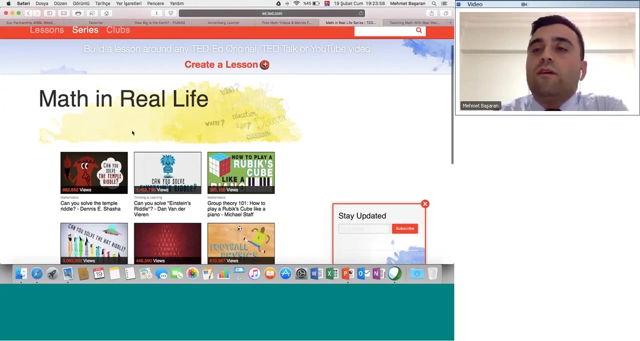 channel. Here you can find some good videos and real-world connection. There are great videos here to use your mathematics lessons. Here are some examples. Do you see? Probably you use them in your lessons, but actually I advise you prepare your own mathematics. 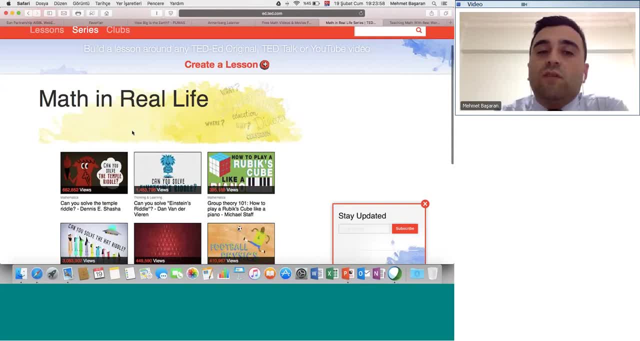 and real-world examples, Because using the prepared one it's more strict. you know, Using them, for example, your own mathematics and real-world connection is very important. So if you like to ask some questions, you can ask me now. 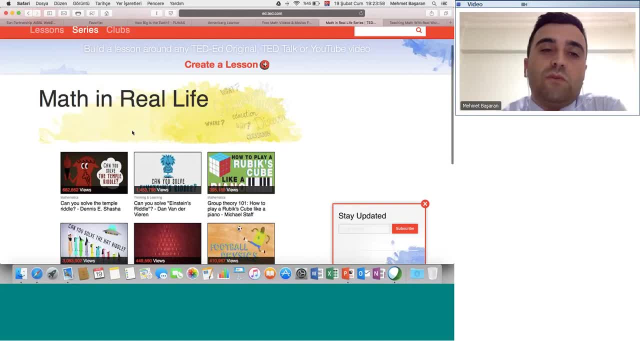 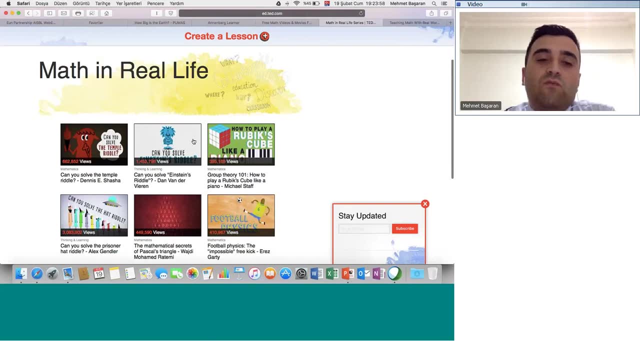 Mehmet, since the websites were not really working in the beginning, if you could add the links that you are using on the chat, maybe this could help people to enter the websites on their own. Yeah, we haven't seen any on the websites mentioned. 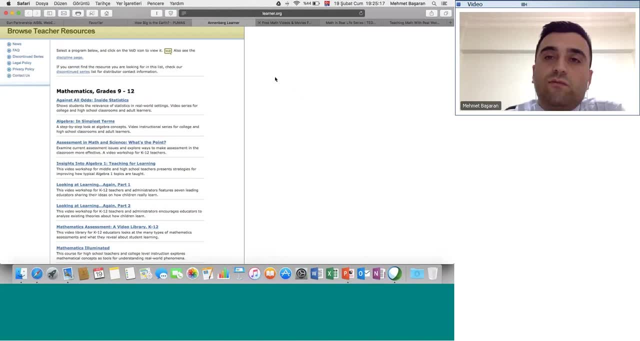 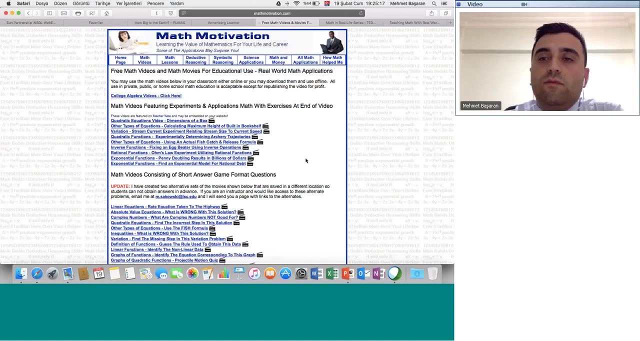 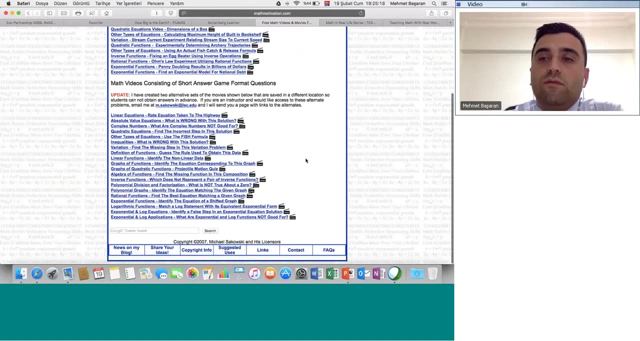 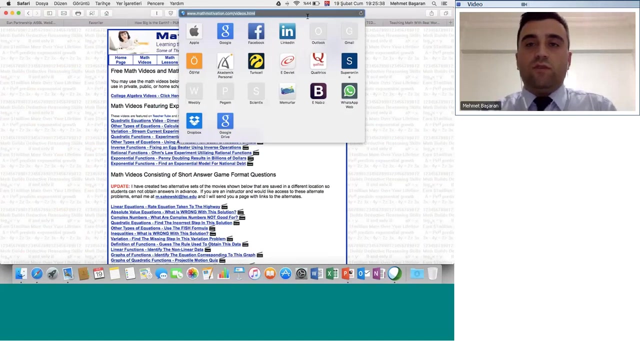 They all seem very interesting, So if anyone has used them or has any comment on them, Yeah, Here are the websites. I copied them on the chat box. Thank you, And maybe we can give a couple of minutes to everyone. So 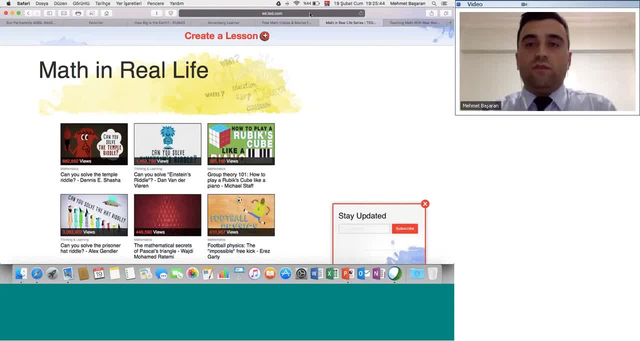 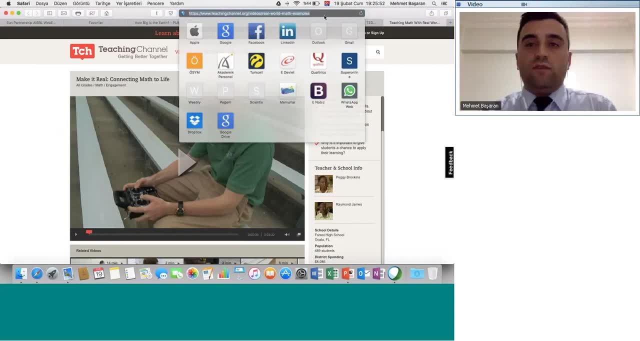 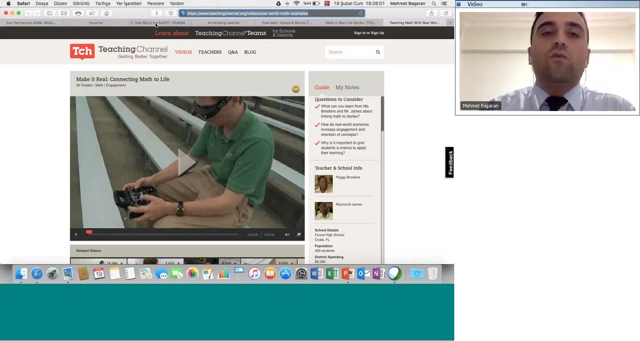 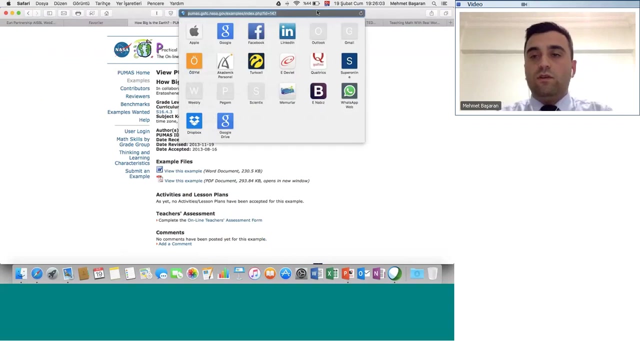 if they want to make a question. Yeah, If you would like to mention about, for example, maybe you use your lessons- the mathematics and real world connections, what are the disadvantages in your lessons? I really wonder such things because I am working. 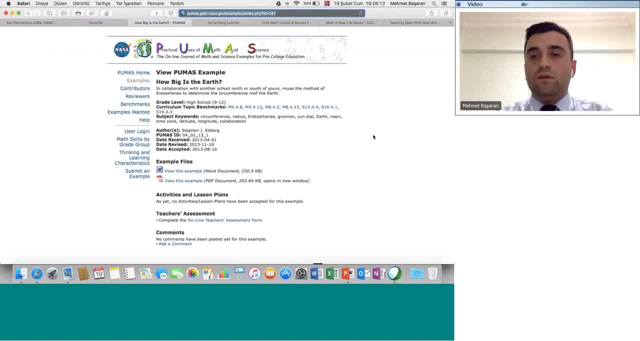 on them. now I am searching the resources from country to country. I know all the things for my country, but actually I wonder other countries If you would like to mention about them. I would like to hear your voice, Okay, So? 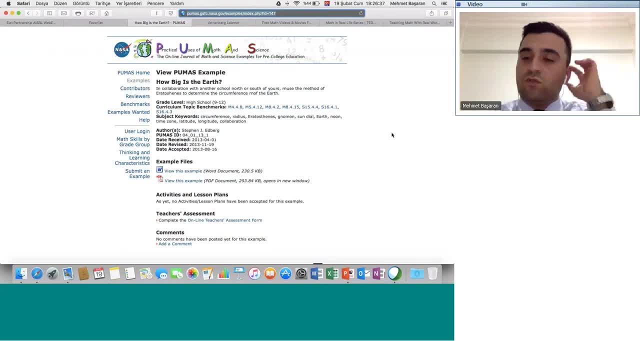 please. if anyone has something to share about their experiences as teachers in their country, please let us know. Okay, For the software from Pumas I use for the software. There is one question in the chat, Liliana. she's asking. 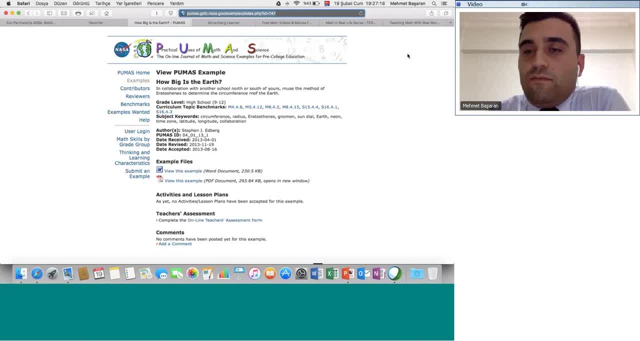 she works with young learners seven to nine years old and she's asking if there's any examples or suggestions for people this age, for students this age. The Pumas are more suitable for students met in real life. Probably you'll see here the 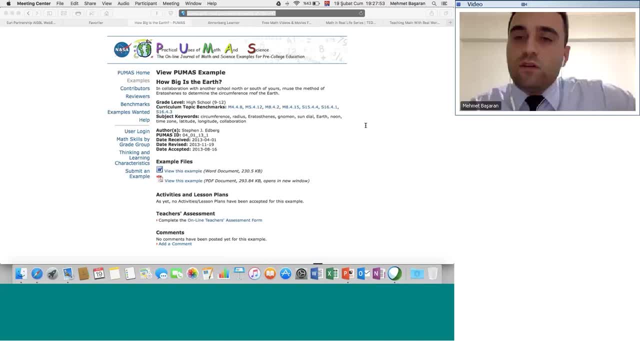 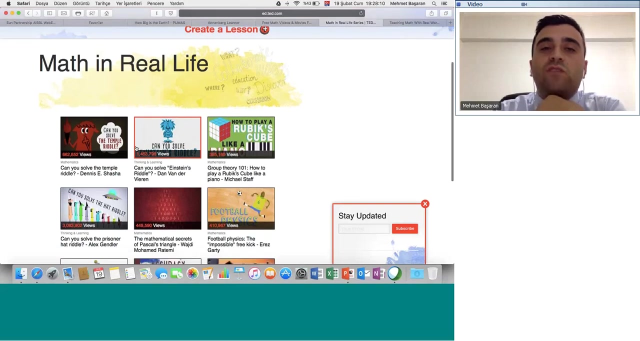 website here at Lessons Worth Sharing. You can use this website for your lessons. There is another comment from Fatih. He's asking. he's saying that the main thing that the research studies say, if you like to use your math and real world connection. 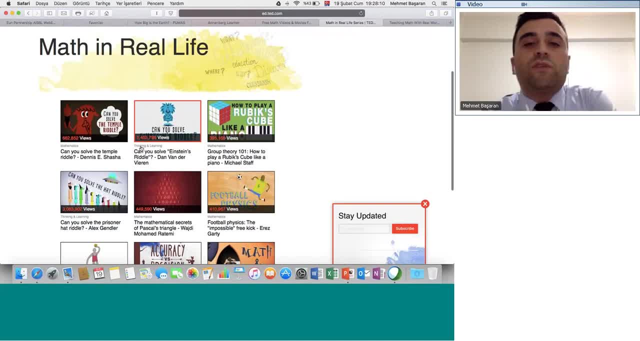 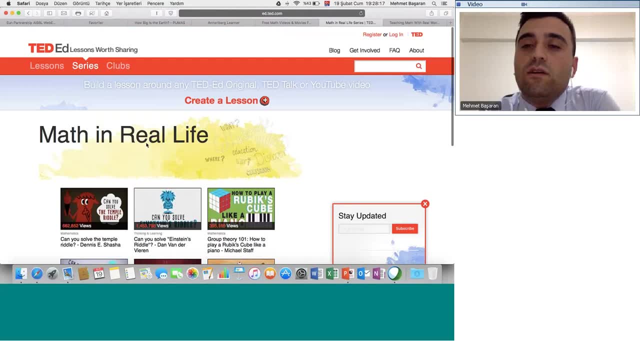 you need to start with small things, For example, giving them to who before the lesson. For example, where do we use the parabolas? Where do we use the limits? Where do we use the differentiation? Just asking such questions is not. 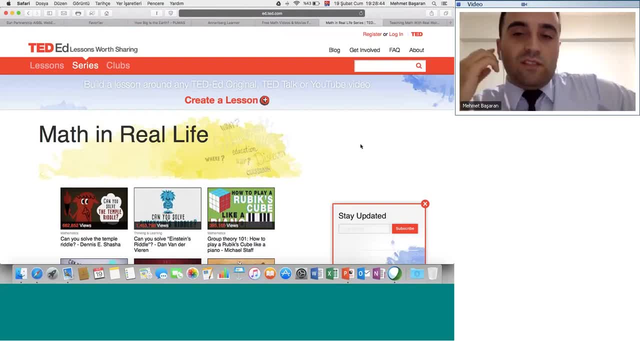 appropriate. I'd like to here emphasize that using mathematics and real world connection is not appropriate for all mathematics topics. I know using mathematics and real world connection is more difficult to use. such for example. the topics, for example say: please use 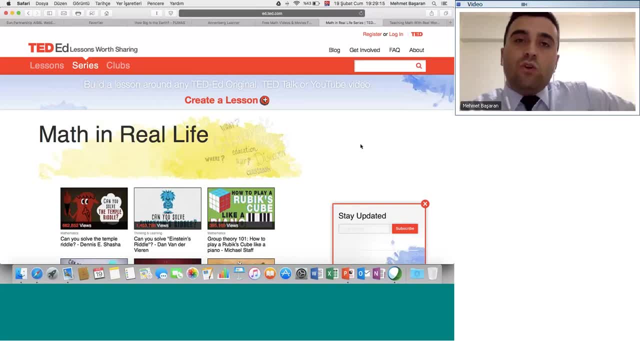 some small things, starting with giving some questions. Where do we use such things in our real life? Have you ever seen before that? Just to hook them before the lesson. After that you can continue. other days you can use some difficult ones. 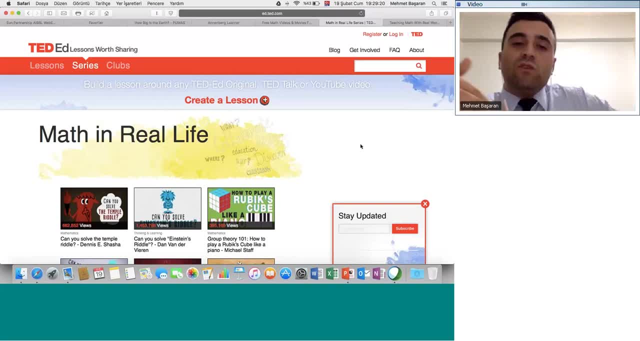 Okay questions. I don't see any other question in the chat at the moment. Oh wait, there is one. There's a comment saying that teachers are afraid of changing traditional methods. Exactly For Fatih. generally it's probably. 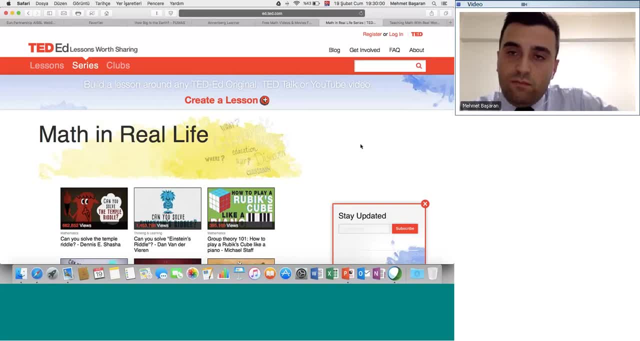 from my country, Turkey. The students must solve different types of problems. Also, the teachers should solve different types of problems. Also, the teachers must solve the mathematics problems quickly, you know, because the students have just one minute for each question. 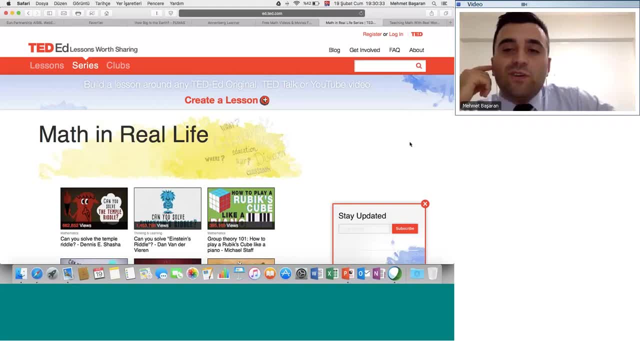 That's why the reason teachers are afraid to change the traditional methods. You know how they can use the technology in their lessons, because using mathematics and real world connections requires some technological content and knowledge. That's why the reason in my country some teachers 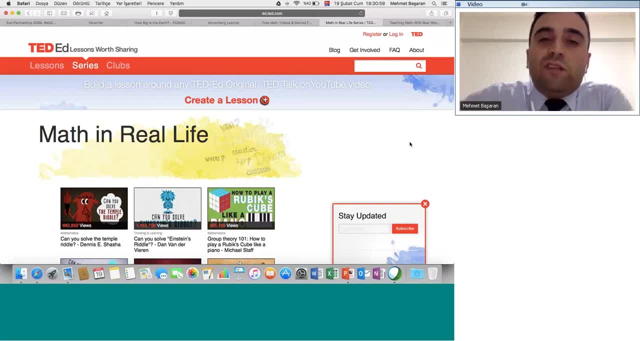 are afraid changing the methods because they don't have the knowledge to solve the problems that the teachers are afraid to solve. That's why the teachers are afraid to solve the problems, because they don't know how to solve the problems. So in IBDP, 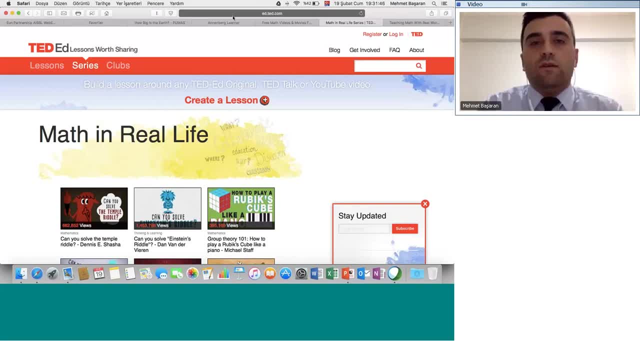 classes. if we use some mathematics and real world connections, students get more high scores in their exams because students must know how to use their TI calculators in IBDP classes. That's why we have some different kinds of mathematical ideas. I actually 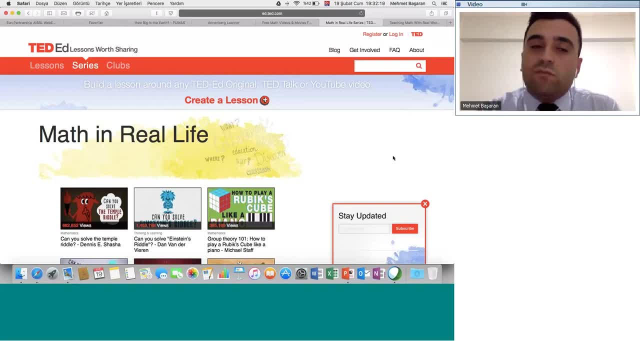 investigated in my MAB classes for Turkey. if we use real world connections, the students get lower scores because they don't know how to solve the problems. So there are lots of ideas in IBDP and in my traditional MAB. 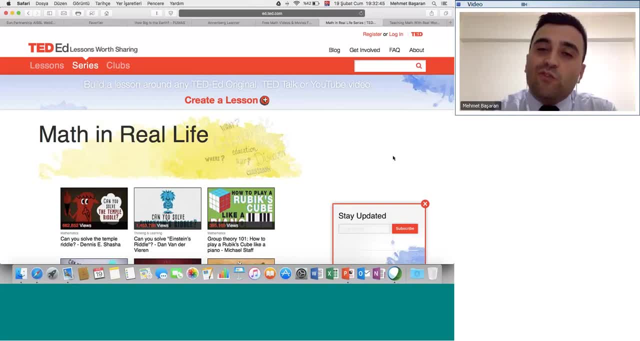 classes is very different. That's why I gave a lot of questions to the students in the MAB classes, So I hope that you have a lot of questions in the MAB classes. Thank you very much for your attention. 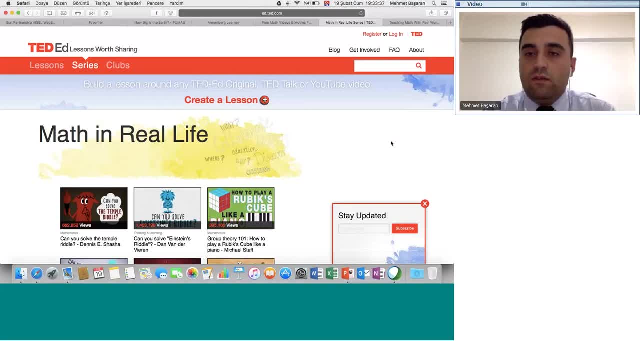 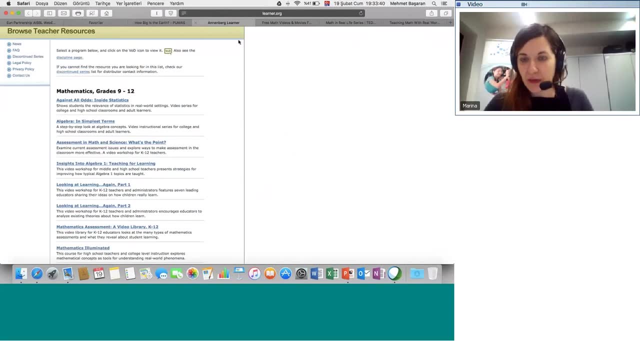 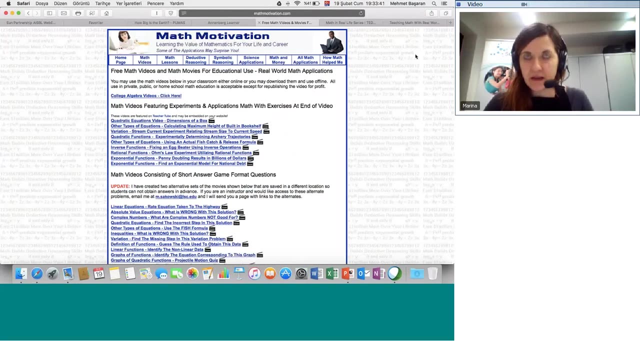 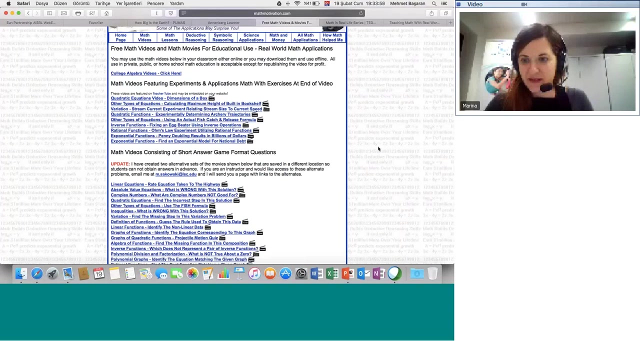 I have another question from Linda Taloya. She was asking for playing games regarding math for 13-year-old kids. And there's also another comment from Katarina Ivanovic. She's lack of materials we can use, you know, if we don't have to use some. 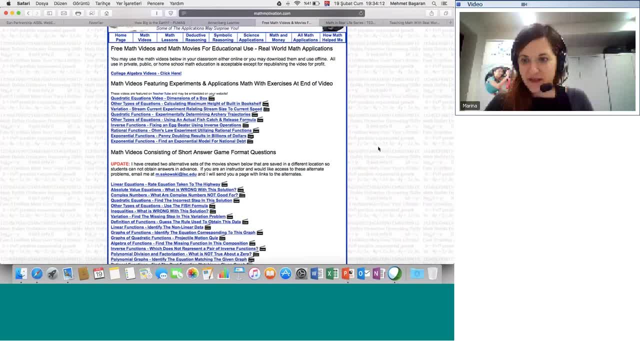 materials to show students how can we connect in real life and mathematics. please try to just show them just one video from the YouTube or other platforms. That will also give chance to the students to think critically. you know, I don't want to advise you. please prepare your lessons, all lessons. 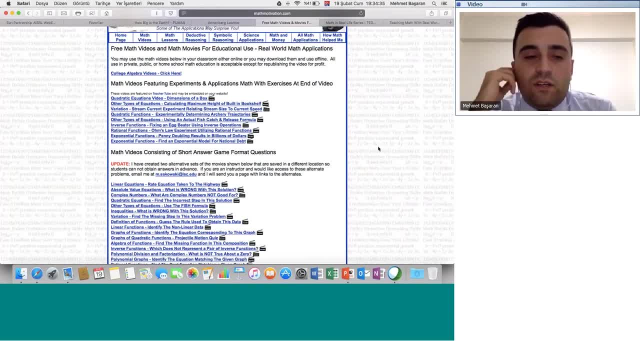 according to the real world and mathematics. That's difficult, but just using some small parts in your lessons using real world and mathematics will give students to think in a different way. you know, If we give them just theoretical knowledge, they will just try to think abstractly. you know. 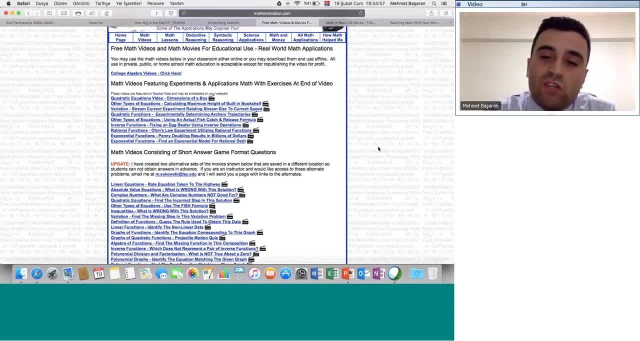 We must consider how can we differentiate our lessons. That's why the reason in the last two decades- this is the research topic and research studies about it- how can we come up with new ideas to teach mathematics? you know They want the students to think critically, analytically. you know many skills. 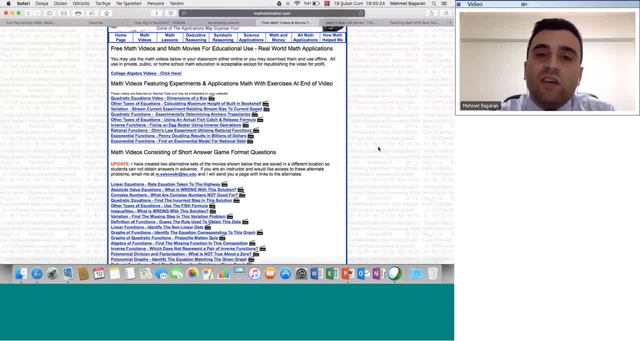 Because the mathematics, the nature of the mathematics, is too strict and too complex. If we try to make it easier for students, it will give chance to think more actively and critically. There is another question from SVEuta. She is asking: what software do you use for modeling? 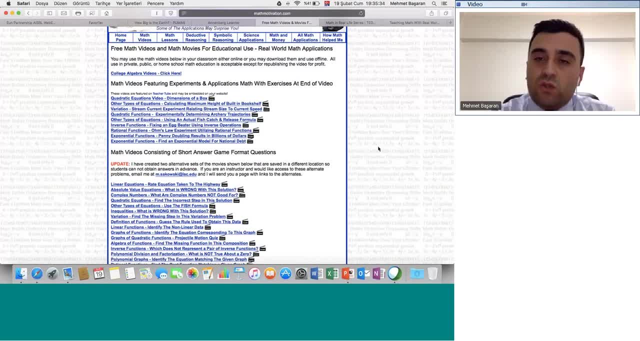 Thank you, Linda. I use for software, Marina, GeoGebra and Phantom, For example, example for my IBDP students. they use TI calculators because it is handled and they can use more comfortably to use their mathematics lessons. And also they use the TI calculators for their exams. One exam: 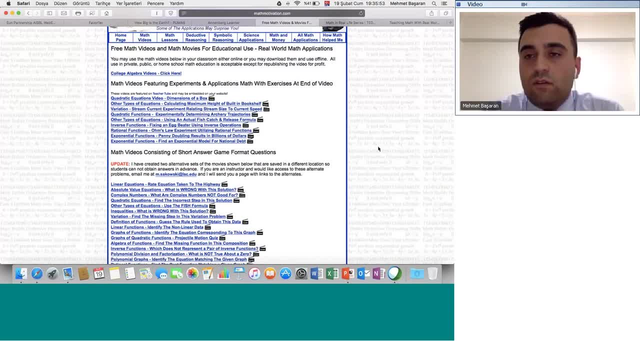 with using TI calculator. one exam without using TI calculator. That's why the reason I want to give them chance to use TI calculator, but for my lessons I use GeoGebra because it gives me more chance to use sliders and other things to make the equations more suitable for my mathematics. 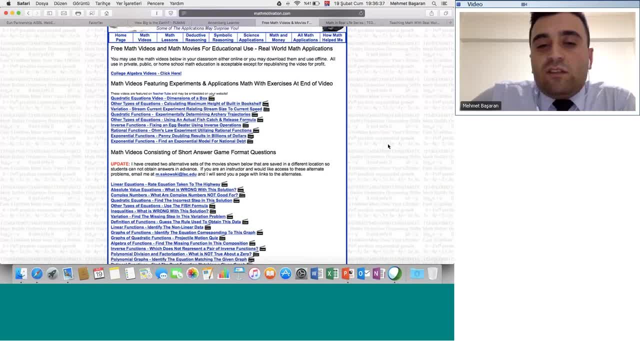 topics. Okay, thank you. Any other questions, please share it on the general chat so we can all see them. Okay, we're going to leave it open for about one more minute if anyone has another question, and if not, we're going to close it. So if you have anything to add, please,